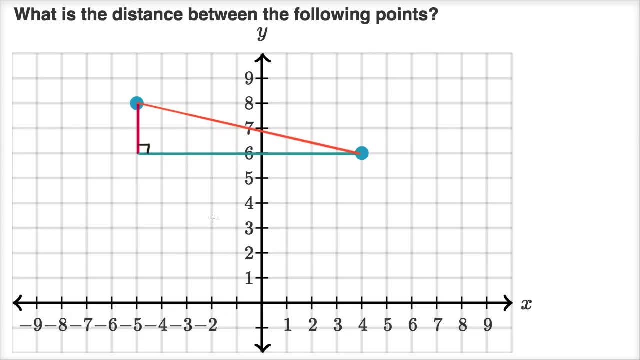 which is the distance between those two points. Well, what is the length of this red line? Well, you could see it on this grid here. This is equal to two, It's exactly two spaces, And you could even think about it in terms of coordinates. 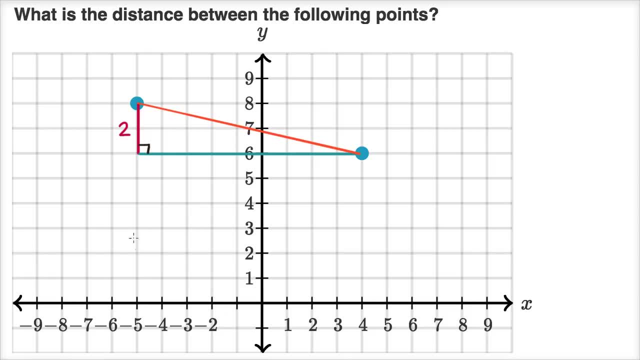 The coordinate of this point up here is negative five, eight, negative five eight. The coordinate here is x is four, y is six, four comma six, And so the coordinate over here is gonna have the same y coordinate as this point. 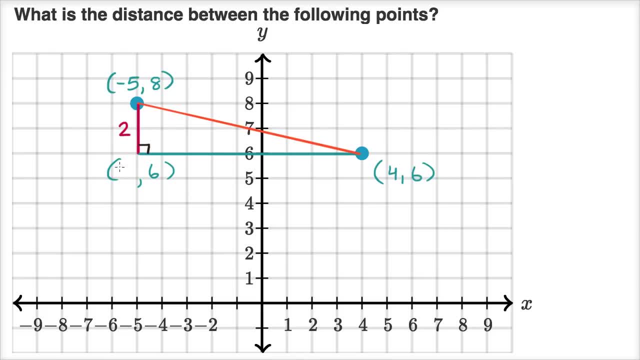 So it's going to be comma six. It's gonna have the same x coordinate as this point, So this is gonna be negative five comma six. And so notice, you're only changing in the y direction and you're changing by two. 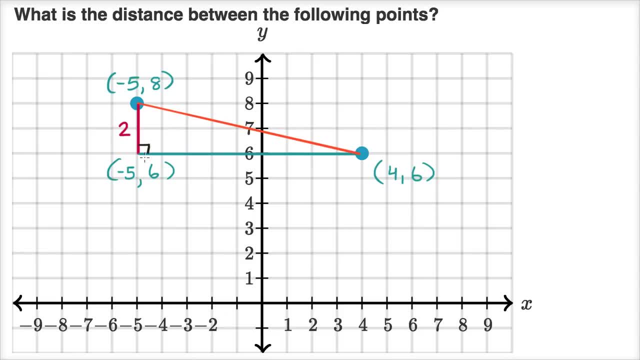 Now, what's the length of this line? Well, you could count it out: One, two, three, Four, five, six, seven, eight, nine, So it's nine. Or you could even say: hey look. 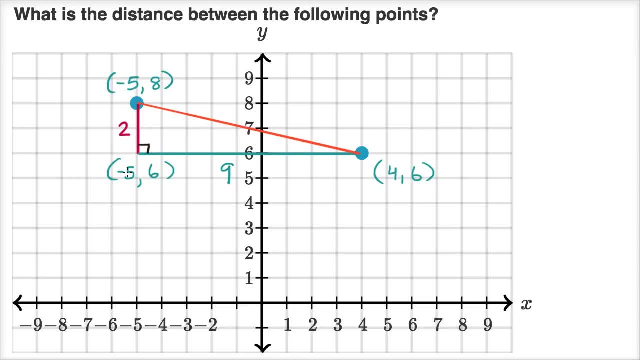 we're only changing in the x value. We're going from negative five- x equals negative five- to x equals four. So we're going to increase by nine. Now, all of that just sets us up so that we can use the Pythagorean theorem. 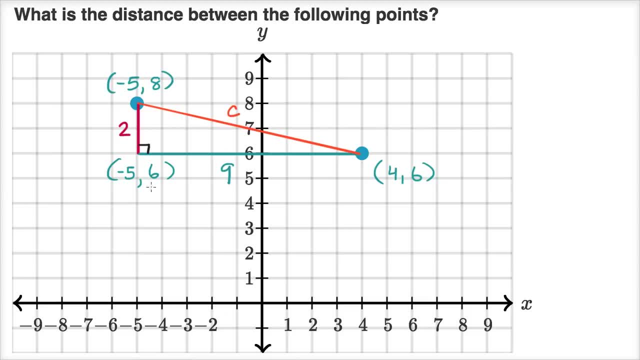 If we call this c, well, we know that a squared plus b squared is equal to c squared. Or we could say that two squared- let me do it over here- is equal to c squared Two. use that same red color. 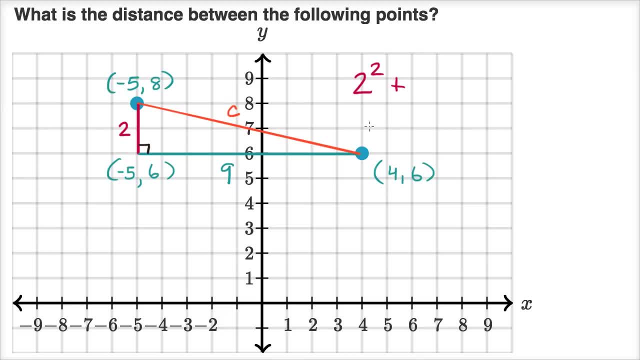 Two squared plus nine squared plus nine squared is going to be equal to our hypotenuse squared, which I'm just calling c is going to be equal to c squared, which is really the distance. That's what we're trying to figure out. 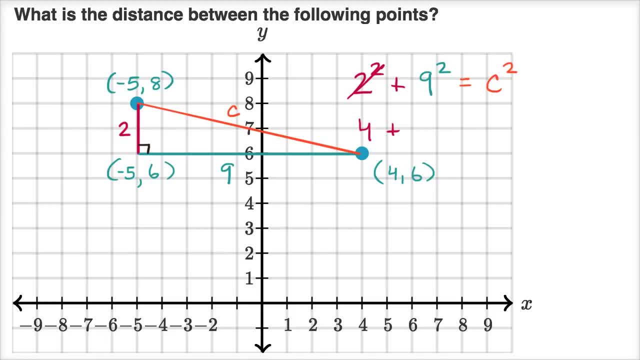 So two squared, that is four plus nine. squared is 81.. That's going to be equal to c squared. And so we get: c? squared is equal to 85.. c? squared is equal to 85.. Or c is equal to the principal root of 85.. 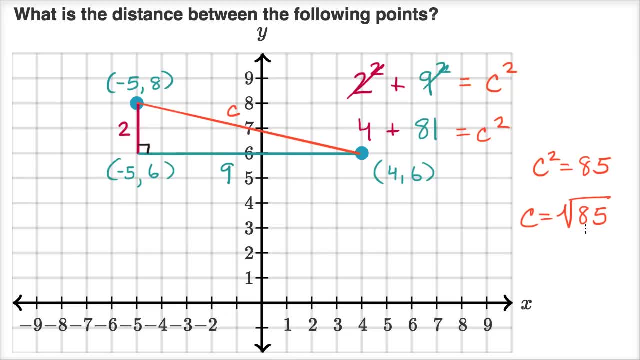 Now can I simplify that a bit. Let's see how many times does five go into 85? It goes. let's see it goes 17 times. So neither of those are perfect squares. Yeah, that's 50 plus 35.. 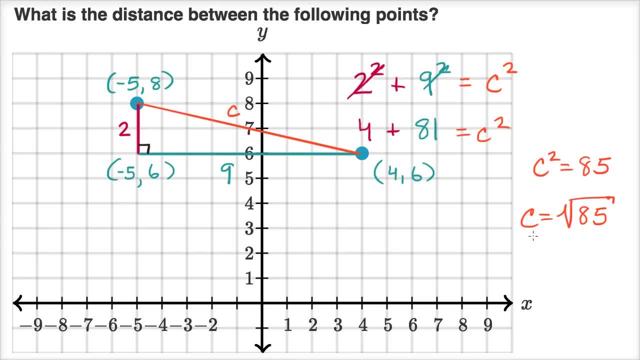 So yeah, I think that's about as simple as I can write it. If you wanted to express it as a decimal, you could approximate it. You could do that by putting this into a calculator and however precise you want your approximation to be, 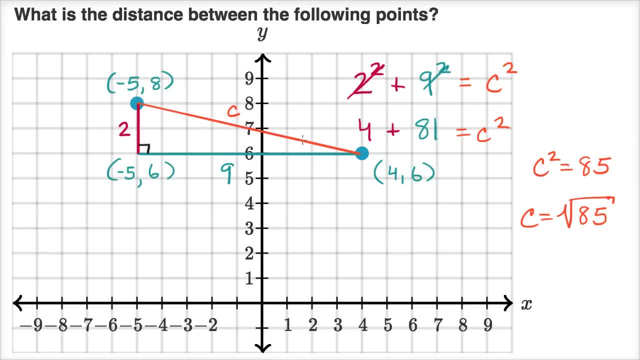 But that over here. that's the length of this line, our hypotenuse and our right triangle, But, more importantly for the question they're asking, the distance between those points. 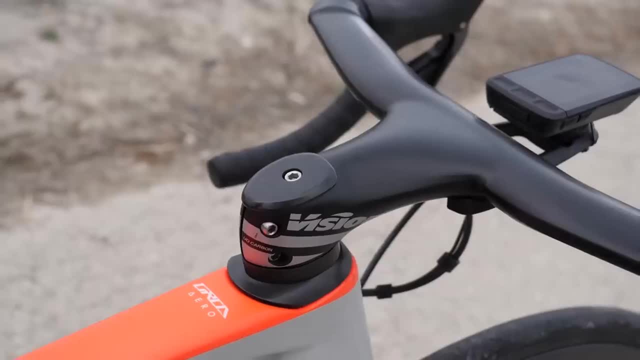 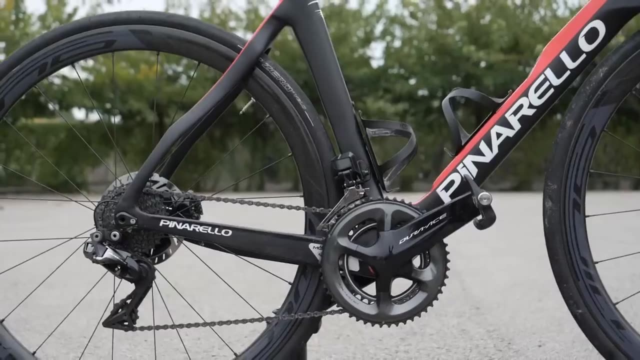 When it comes to buying a new bike, it's absolutely paramount that you pick the right size. There are loads of different adjustments you can make to your bike, like the stem, the saddle, even the seat post or the crank length, but every different adaptation you 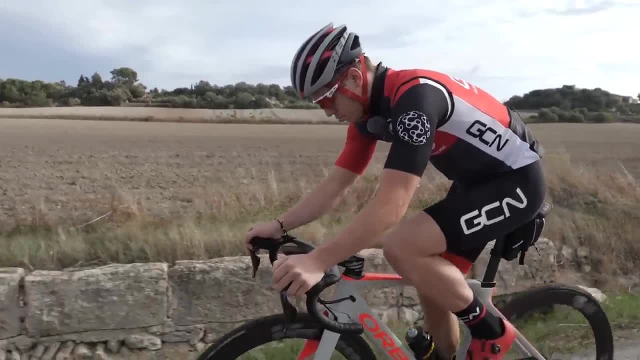 make to your bike will affect the way it performs and the way it feels. Ultimately, if you're buying a too small bike, or even a too big bike, it's never going to feel quite right. In this video, we're going to help you choose the perfect bike size for you. 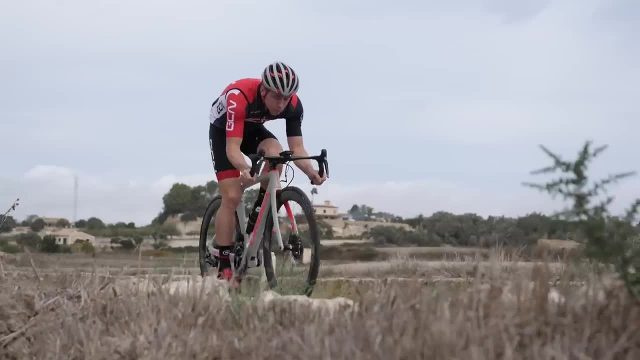 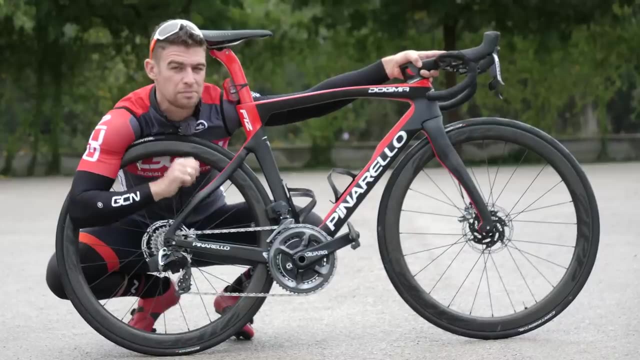 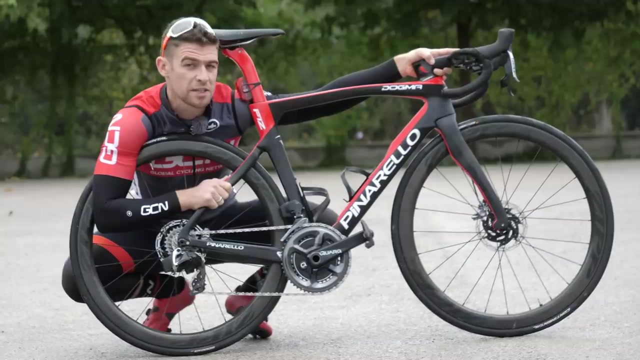 Before we start, let me explain sizing, because it's not quite as simple as just basing the bike around- how tall you are. Most manufacturers will label their bike in sizes small, medium or large, et cetera, but others will also label them with a number. These generally range from 48 to 62,. 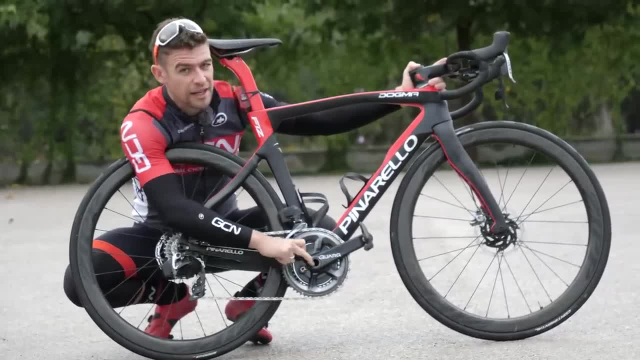 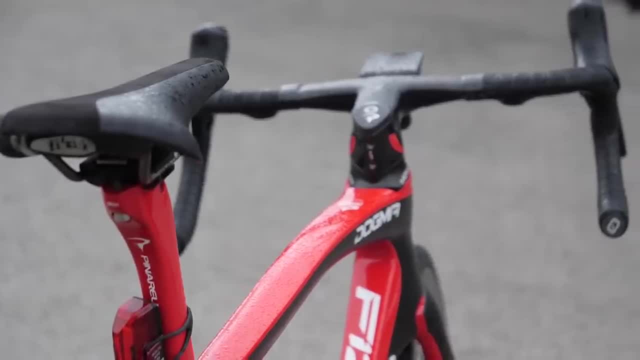 and that corresponds to a measurement in centimeters from the bottom bracket, which is down here, to the top of the top tube. There is, however, nothing consistent about the way manufacturers make their bikes, Just because you've always had a 54 from one brand. 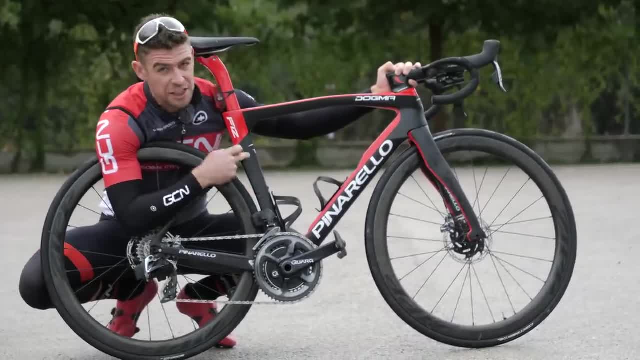 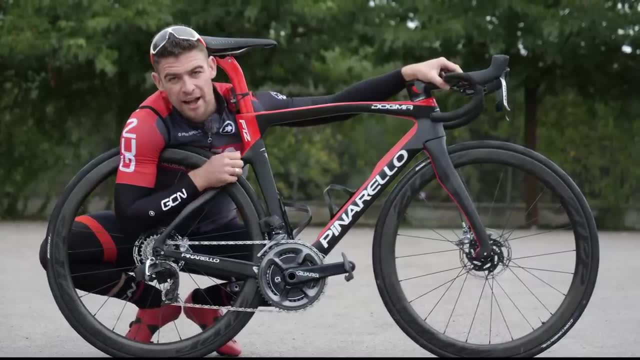 doesn't mean that a 54 from another brand will fit you. The effective seat tube length is just one of three really important ways of measuring your next bike. The other two ways of measuring your bike are known as reach and stack, and these are internationally regarded standards. The reach refers to a centerline from the bottom.